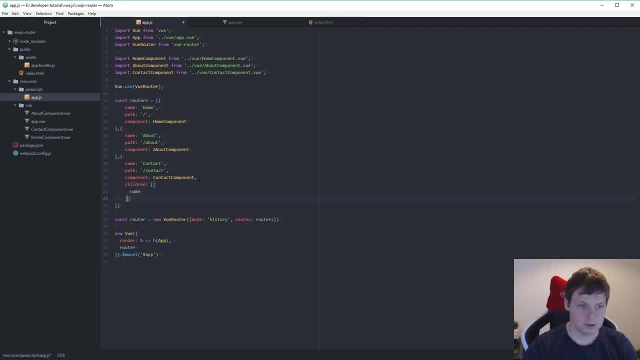 and we have a name On a contact I don't want. I don't want It's here, It's destroyed a little bit of my claim, So we move it up here on about- And in this case I will call it about me And the path should be me And the component could be anything, But I don't. 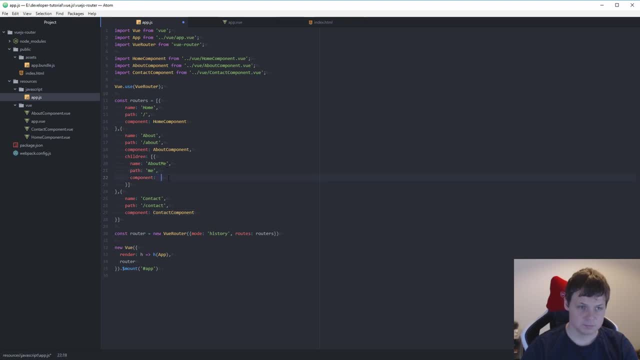 want. I will say about me component And then we copy it One more because I want one page for my dog And I call about dog, Dog And dog. Then we need two new components: Dog And me. Let's copy the about. It should be me, Add this and this And go back and say about dog. 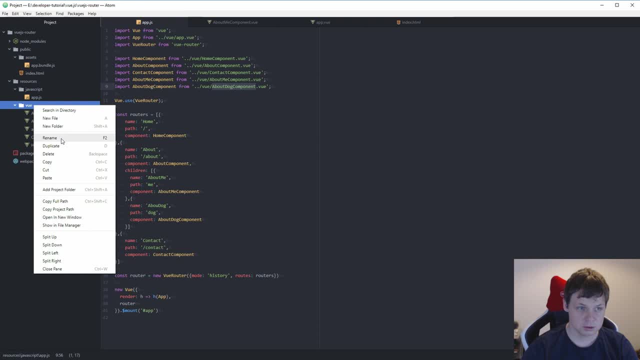 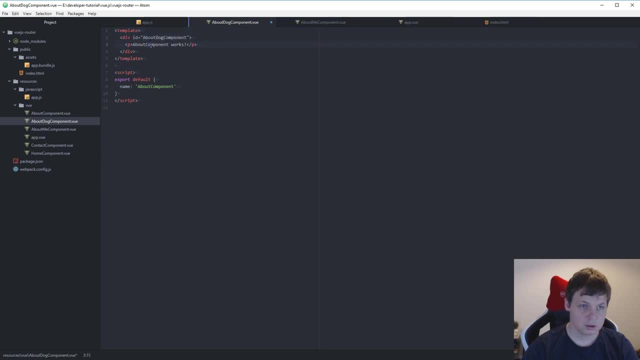 And about page here. Duplicate about dog. It's here, And then you need the yes and then we need to go to this one. I need to move So it's checking from the route and not from the page URL, because now we are going a level deeper And then I need 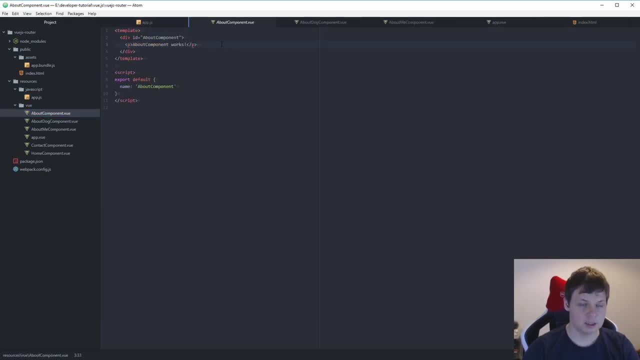 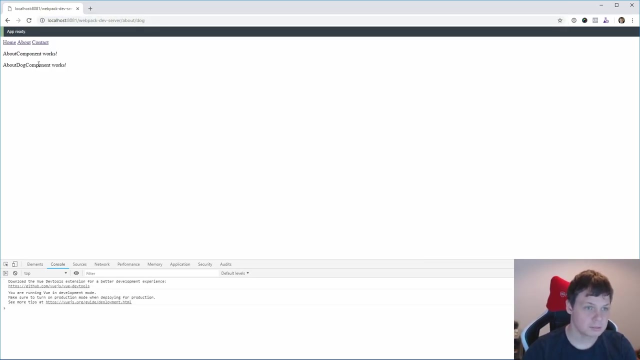 that about here. I need to say: here it's the router view, Here router view, and that's it. if I open my my about me, you can see about me and I can say: my dog, it's my dog and as you say here, but you can see it's no.